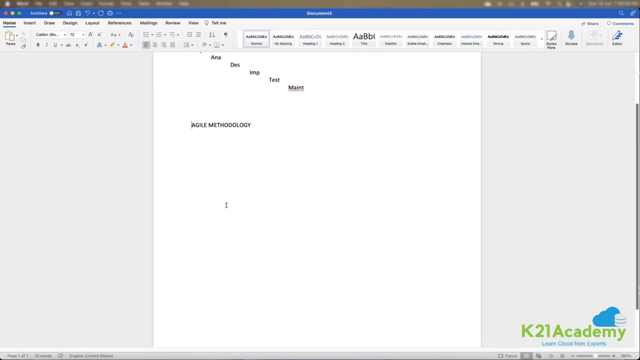 inside an agile methodology is still the same, which means here also I'm just going to do a: requirements gathering, analysis, design, implementation, testing and then maintenance. the process is the same, but I will be doing it in an regular intervals of time, which I call it as an iteration, alright, so 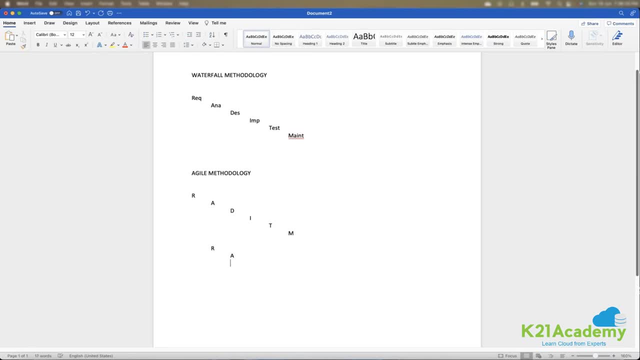 every iteration, right? I will just follow the same process. and every iteration means it is at least two weeks to four weeks to six weeks, so, depending upon the time frame, right? so I will just do the same iteration and the same process for that. at the end of this process, I will just follow the same process and then 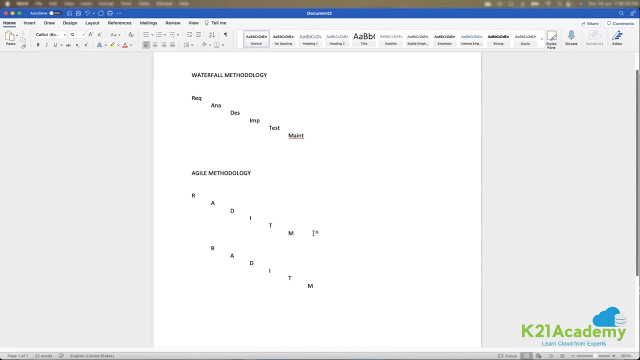 the client will be able to see the result at least after four weeks, and after four weeks if he is not satisfied or if he needs any change, immediately I can take that change and then I can pass it on to the next requirement and immediately after next four weeks I can show that to the client. so the client 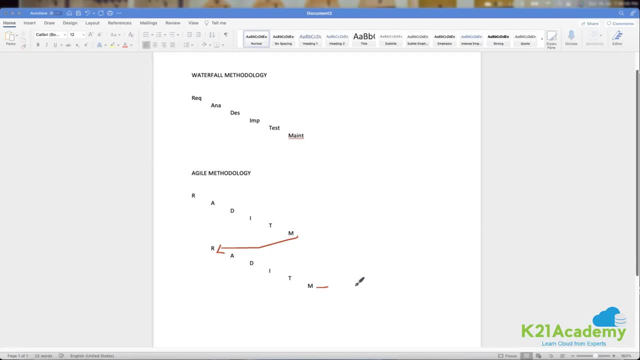 and the company is always connected to each other and the feedback loops is always happening from the end customer, so that the end customer is also satisfied on what does the work we are doing and at the same time we can also cooperate with him to give the desired result of his needs right. so that is one. 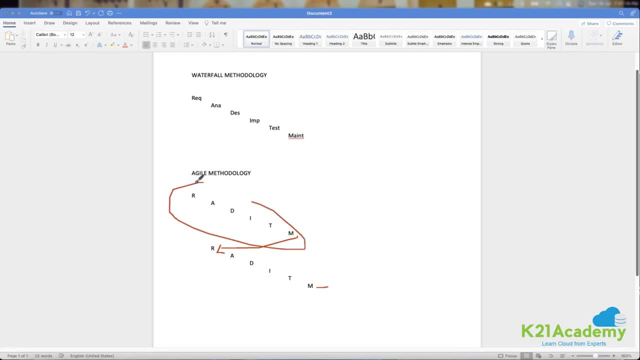 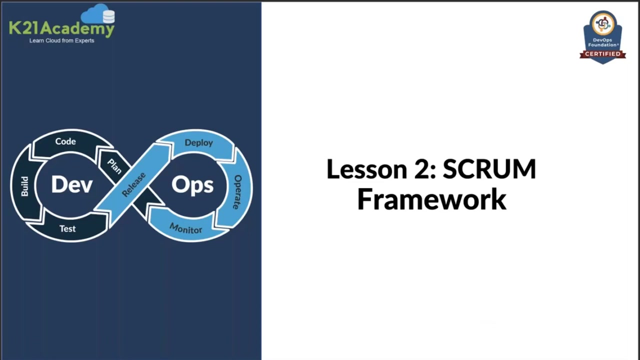 of the advantages of this agile methodology becoming very, very famous in this modern situation. right, so this is called as agile methodology, right so most famous framework of agile is scrum, because crumb is actually followed by 90% of the world companies. right, and in that's why scrum is very, very important framework that is mainly successful for any software. 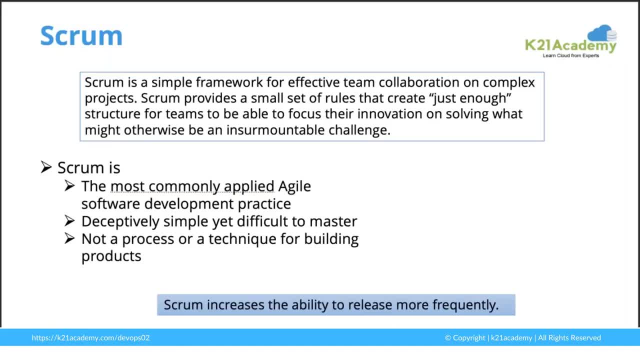 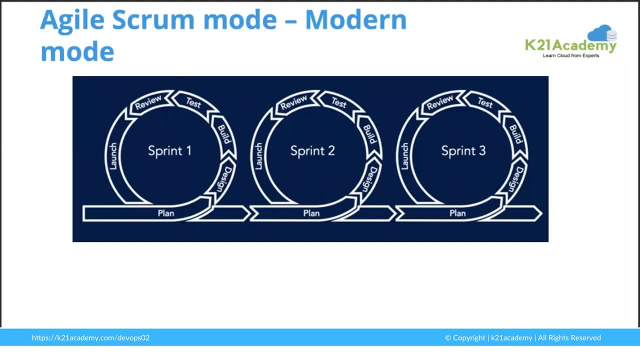 development. right? what exactly is a scrum? scrum is, again, as i said, it's the same process of agile, but you're just going to do it on a regular intervals of time. so you're going to do the same requirements- gatherings, analysis, design, test, implementation and maintenance- but you will be 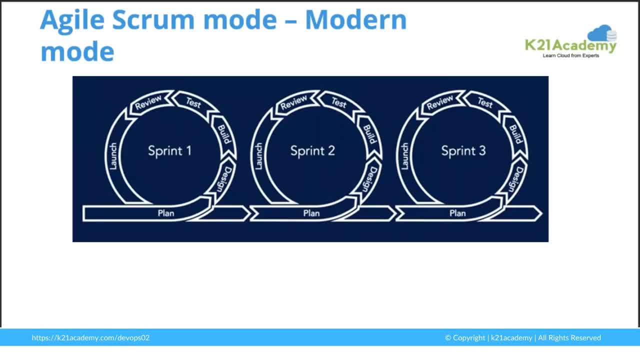 doing it in a regular intervals of time, so that regular interval you can call it as an iteration, or in scrum we we call it as a sprint right. so every sprint will be four weeks to six weeks or two weeks to four weeks. it depends upon the projects or depends upon the client right. but 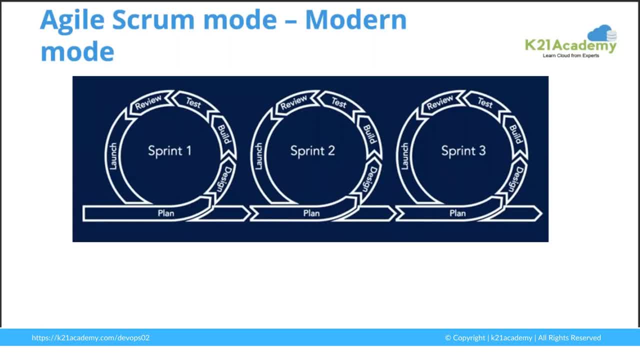 not more than six weeks. so that is how a sprint will happen, and every end of the sprint you will have something to show it to the client and that is called as an mvp, which is minimum viable product, at least a basic result or some dummy web page you have to show it to the client, which we call it as. 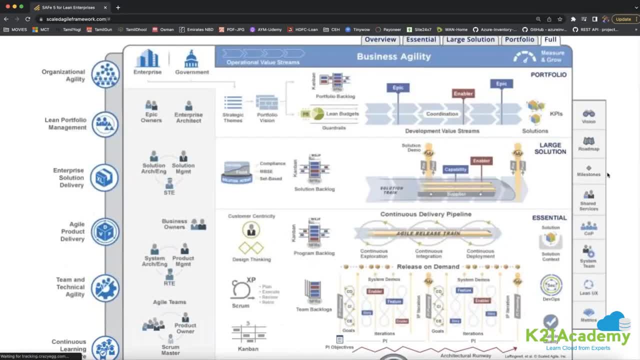 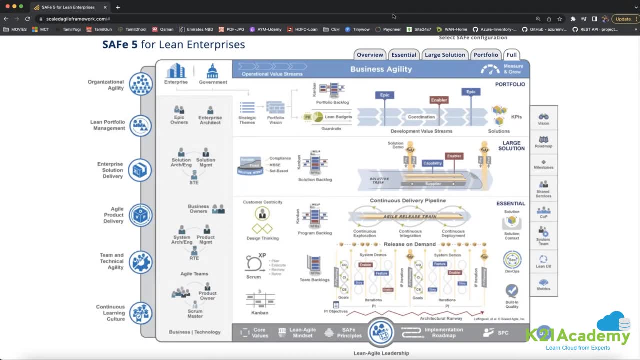 mvp for the particular sprint. you see, this is my scaled agile framework, so this can be applicable only for enterprise companies or government companies, which has more than 500 to 1000 people. right, the one that we that we are discussing is only on the bottom, most level. 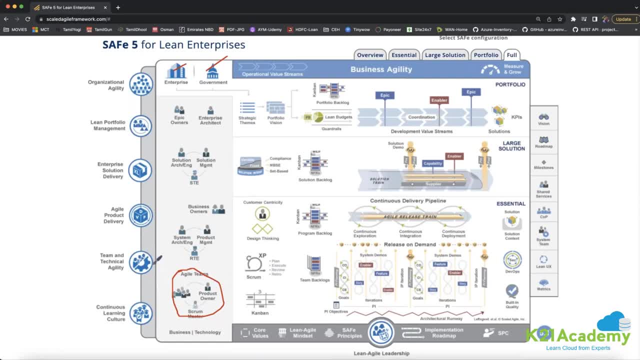 where you have only 30 to 50 to 70 people, so your company, where you implement your sprint scrum, will end here itself right after that. if you have more than 100 to 200 people, then comes your next step, where your release trains and everything will come in. 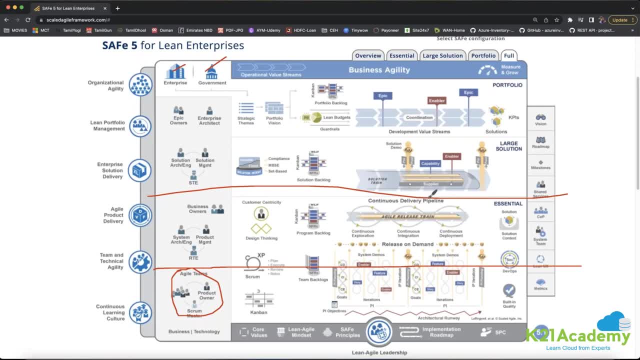 right. so after that, if you have more than 300 people, then comes your next stage, which is called as my solution train, and then here is where your main c-level groups will come in, and the c-level groups and the business, the decision makers, the financiers, everyone will participate. on the last level, which is called as 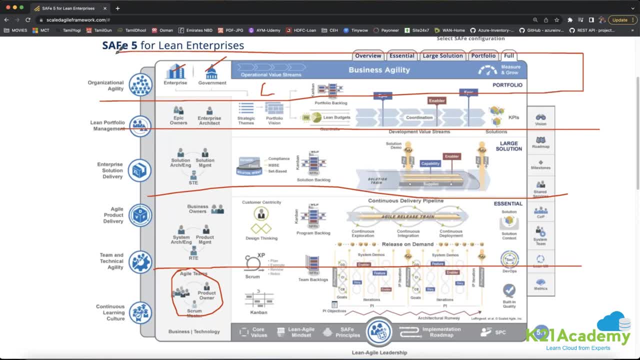 my operational value stream, right? so these many layers you have on implementation of a safe, okay, so let me explain you in one level, detailed one, right? so here, whatever we discussed till now on a scrum and other things, I told you we have something called as scrum master, right this? 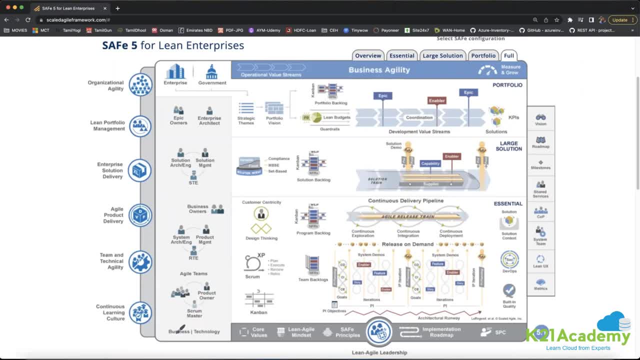 scrum master. this scrum master will be handling a team of maybe 10 to 20 people, right, and here itself scrum of scrums will also come. okay, now I have more scrum of scrums of scrums, which is I have more than 100 people, then what will I do then? all these 100 people will be reporting to one person. 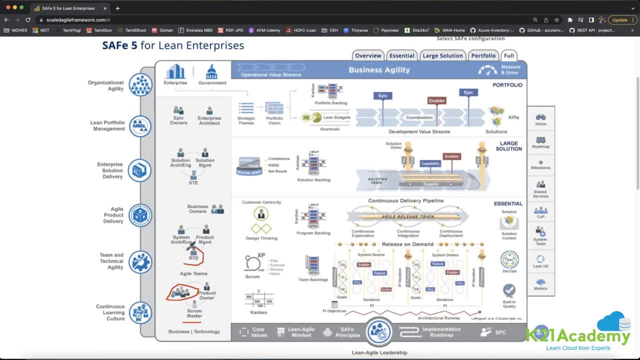 called as RTE, which is release train engineer. okay, this release train engineer will have more than 100 people reporting to it. in that 100 people, you will have multiple scrum of scrum of scrums masters plus scrum of scrum masters plus scrum masters plus team. okay, so this RTE itself is a very powerful role in 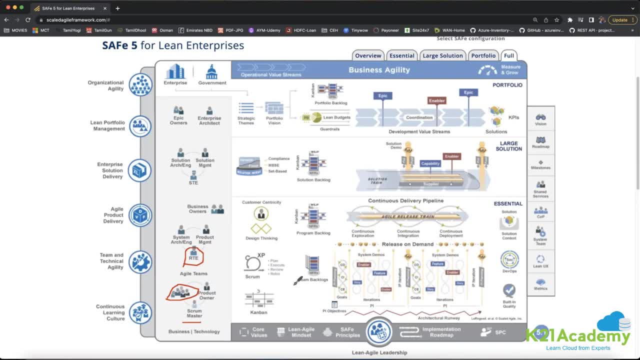 safe because he is the one who is determining the multiple scrums and how a release train should happen and how many deliverables are happening and other things about right. so this RTE is a very, very powerful role in safe. okay, next, multiple RTEs, okay, one RTE itself, as I am. 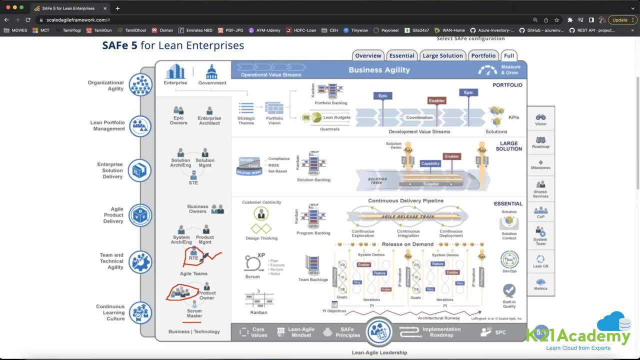 saying, 150 people- okay, multiple RTEs are reporting to one person called as STE, which is solution train engineer. then imagine how much powerful the solution train engineer will be. okay, and multiple STEs will be reporting to someone called as epic owners. then these guys are very, very powerful because they are belonging to the C level. 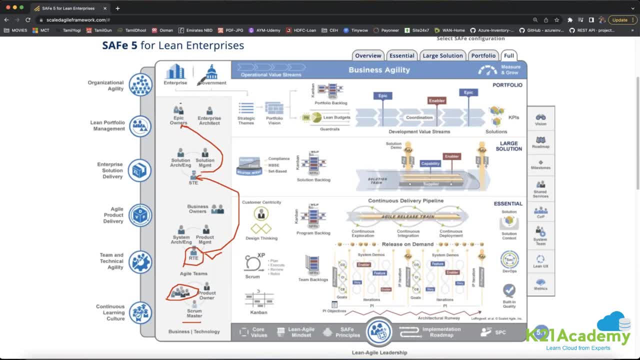 and this epic owners and enterprise architects will be directly reporting to the CEO. okay, this is how the structure of safe will be. okay, now this RTE will be reporting to the CEO. okay, and multiple RTEs will be reporting to someone called as epic owners. determine what is my current sprint. how long should I take for this product to be delivered? 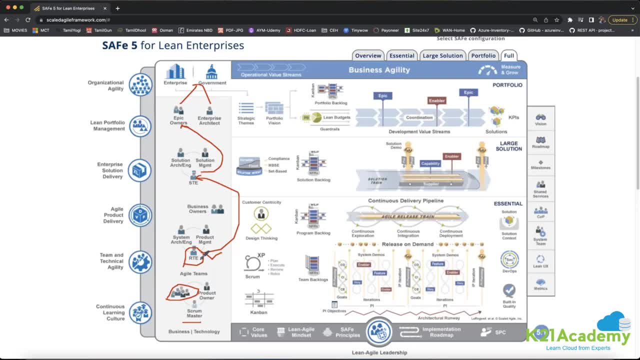 is it six weeks? okay, in this six weeks, multiple teams- maybe 10 scrum teams- will be working together to deliver a product in six weeks and that process is called as ART, which is agile release train. okay, some of our colleague also said something called release train. 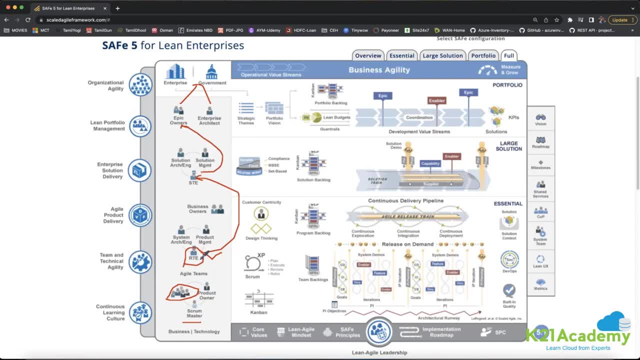 right. so what do you mean by release train is nothing, but it's a sprint, okay, in safe we don't call it as a Sprint in safe, we call it as a ART, which is agile release train. so where is my train taking? from one destination to another destination. that is the reason it is called as released. 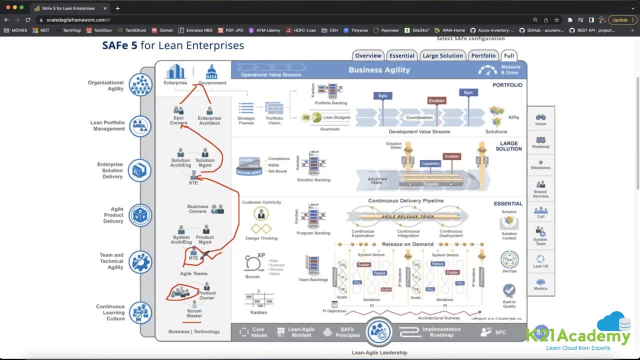 train right. so that release train and the release features and how long it will take, how many teams has to participate, everything will be decided by this RTE. okay, if suppose the ART, which is agile train, is not getting delivered on time and it is getting failed, only then this: 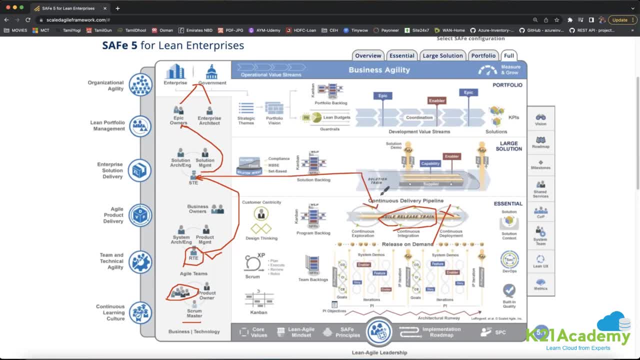 guy will come into the picture, which is STE, a solutions train engineer will come into the picture only when my ART is getting failed. then what he will do? he will take this ART under his control and then he will form something called a solution train. okay, he will be including his capabilities, his enablers and other. 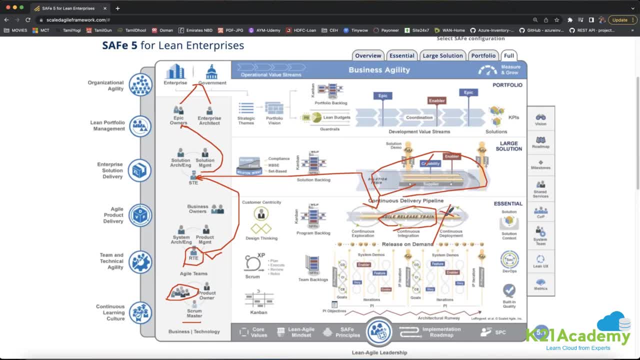 things and all, and then he will try to make this failed ART into an solution train and he will deliver it to the customer. okay, if this ART and SRT, which is solution train, is also getting failed, only then this enterprise architect and epic owners will be jumping into the picture. if not, these people and all will. 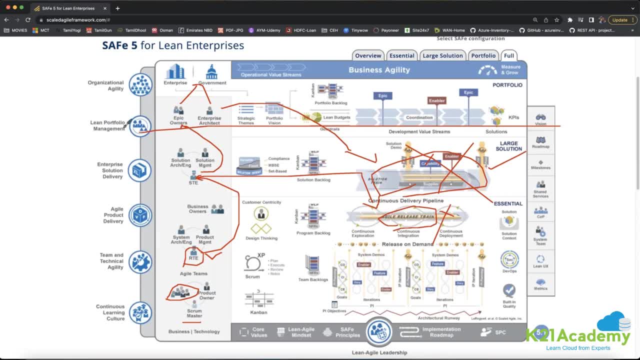 not even bring the solution train into the picture. if this ART and this solution train is not even look down what is happening, these entire portfolio management will be only visible to the CEOs. they don't even know what is happening on the underground. okay, these people will only come. 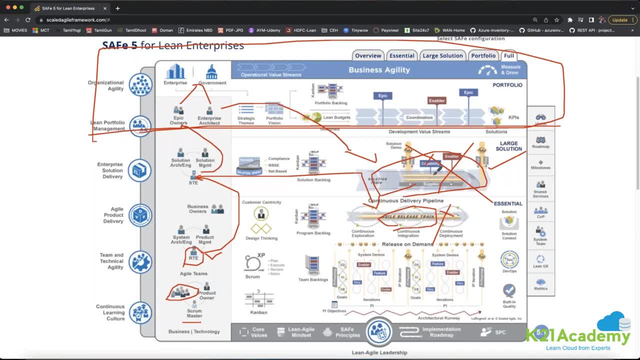 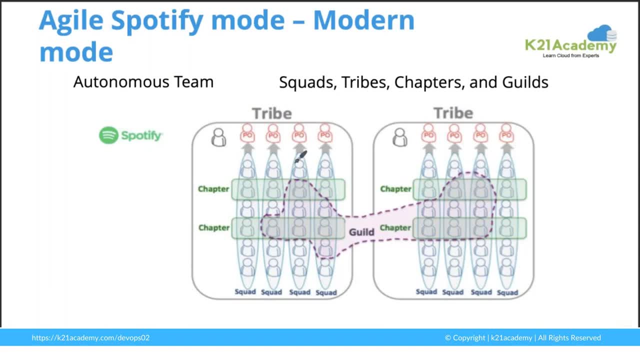 in when there is a multiple failures on ARTs and SRTs. so this Spotify- we call it as agile 2.0. okay, some companies have started adopting it from 2021 onwards and now, by 2022, a lot of other companies will also implement this agile 2.0, which people call it as Spotify model right. 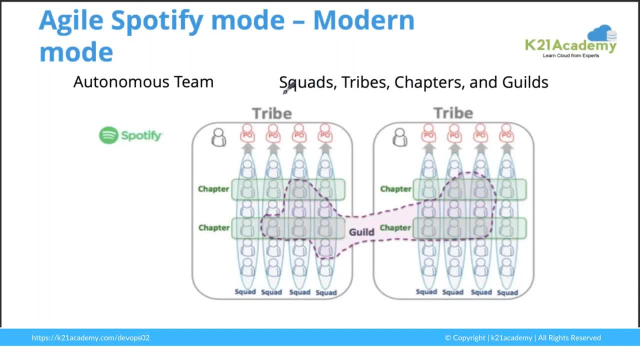 so what it is is like I have two different projects, so this is my project one and this is my project two. okay, so on a scrum team, I would say on an agile team, you will have a developers, you will have testers, you will have database guys and you will have maybe unix or whatever guys. it's right same. 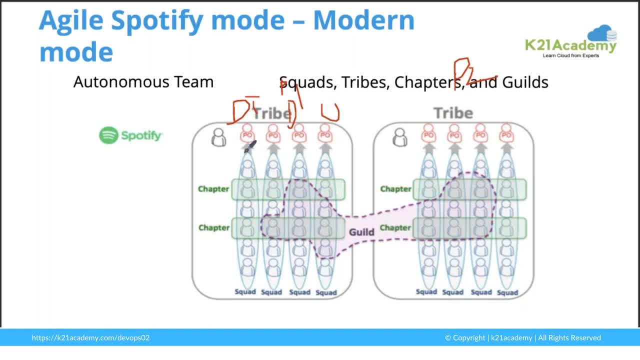 for other scrum teams and other things. so combination of all the developers together in a particular project is called as my squads- okay, combination of the scrum teams together is called as my chapters- okay, the entire project. people is called as a tribes, and picking up the best of best people and then forming a special team is called as my guild. 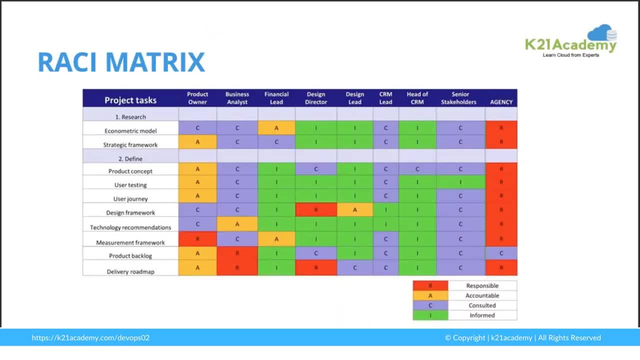 that's what is agile 2.0 during a starting of the project, right? so there will be a collective decisions and they will be coming up with this matrix. what are all the different task items? what are all the different team? what are all the different team members? 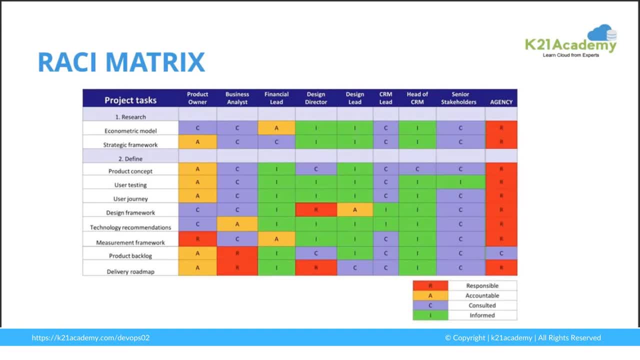 what is the role for them, who are all responsible for this to deliver, who are all accountable for this to deliver, who are all informed, who are all consulted. so this will be done during the initial project discussions and starting of the projects, right? so, on a nutshell, I'll just tell you what are all these four items right, responsible in the sense. 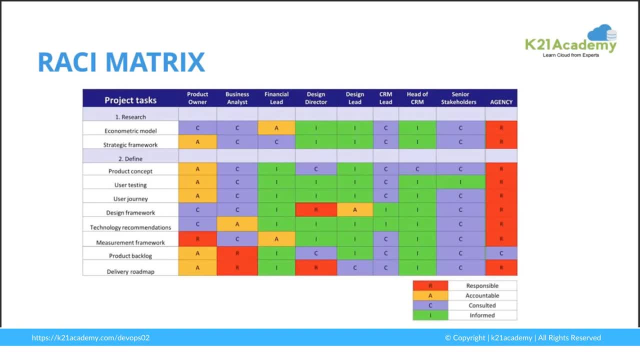 you are responsible to deliver it, no matter what right. that is what is called as responsible for. so, for example, if you want to deliver some website, then I don't care how you deliver what you deliver, but you are responsible for delivering it, so you have to deliver it. no other option. that is responsible, accountable is nothing but. 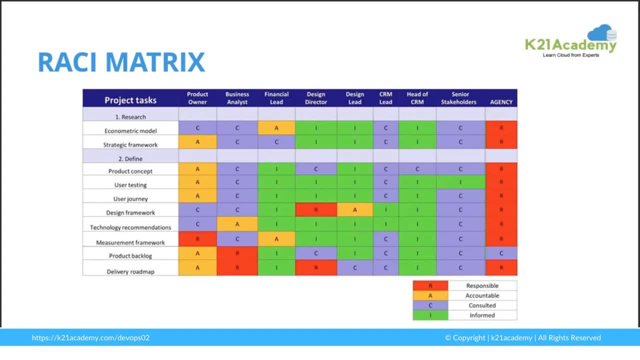 you are required to deliver it, but I don't care whether you are going to work it or someone else is going to work it. but you are accounted for. if the project is not delivered, then I will be holding you accountable for right. but I don't want you to work or I don't want someone else to work. that choice is given to you. 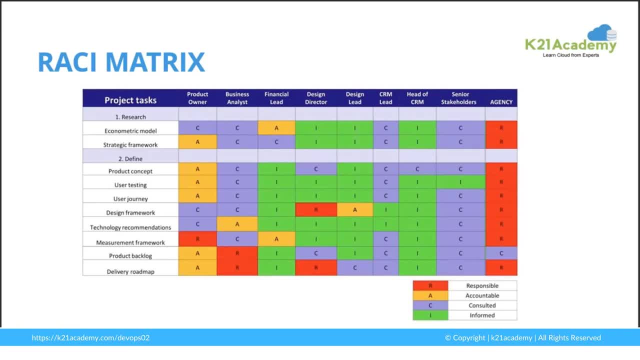 right, so that is called as accountable. consulted is nothing but an SME, right, so the subject matter experts. if you get stuck in something else, then you can talk to the subject matter experts and get the consultations out of it and and then solve it. that is consulted, informed is nothing. 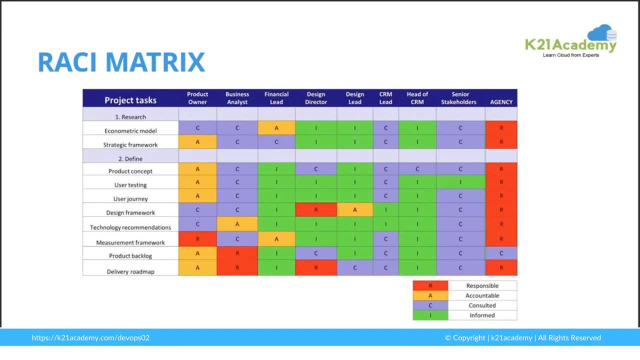 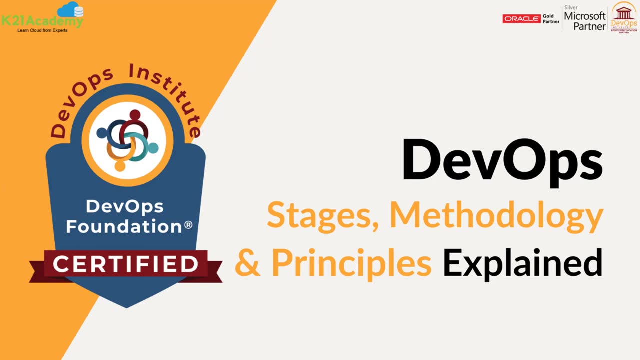 but keeping someone on the cc just to inform them like something is going on that is called as informed right. so these are all the four main items on this particular aspects of RACI matrix right. so, guys, this was our expert from team k21 academy and if, in case, you missed upon anything or